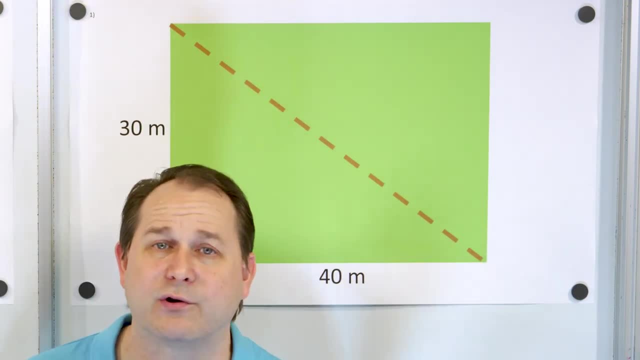 by 40 meters. question is: how long is this? Now, this is very practical. This is a real life situation. Now, you could guess that it's going to be a little bit longer than 40. And, of course, it's going to be longer than 30. And so you could probably go to the store and buy 50 meters worth. 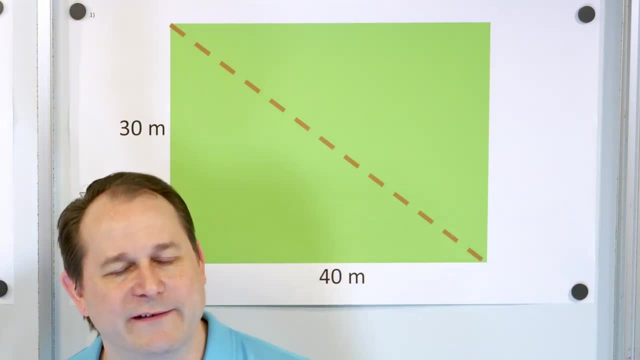 of material, but you might not have enough or you might have overpurchased, And it's just better to calculate what we need. So let's treat this as a problem with the Pythagorean theorem, because, you see, this forms a right triangle here. Of course, this is a right triangle here. 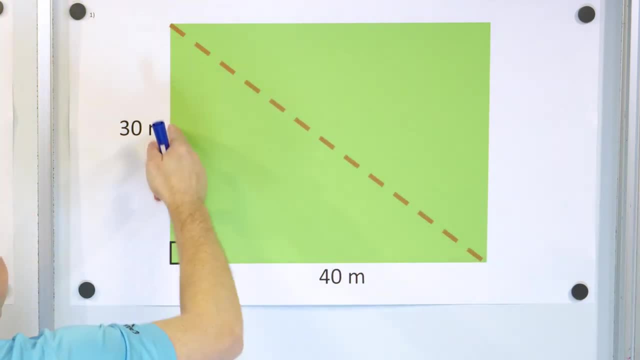 And the diagonal that you calculate here is exactly the same length. So we're just going to focus on this bottom triangle here, And we know that a squared plus b squared has to equal c squared. Now, a and b are the sides of the leg of the triangle And this side right here. 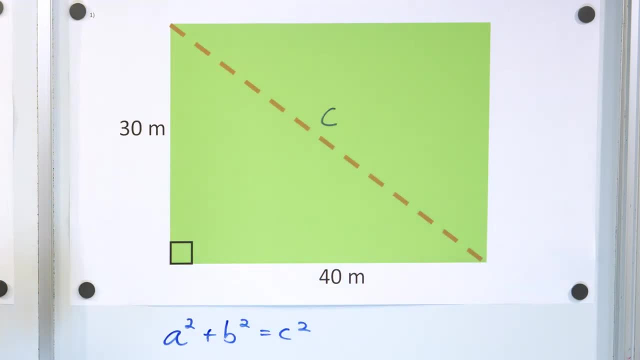 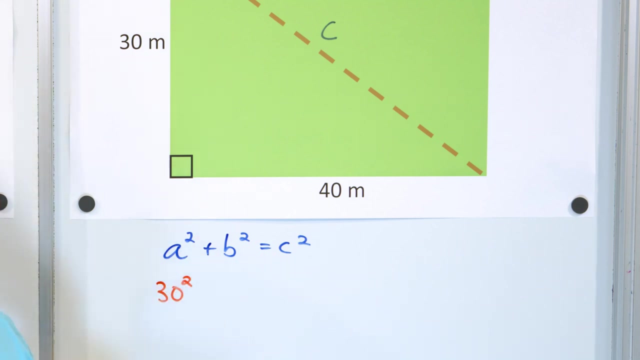 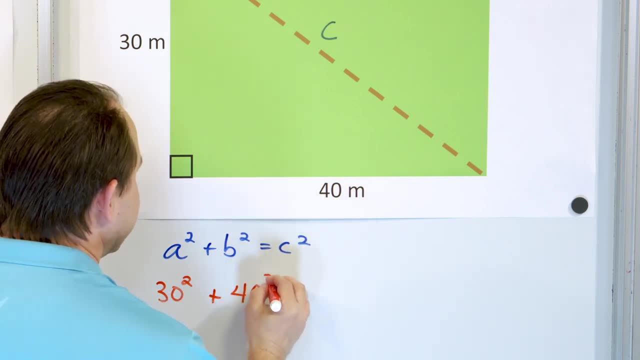 So we know that b is going to be 30 meters- We're not going to put the units in here, but we know that it's meters we're dealing with- And then b is going to be 40 meters, So we'll put that 40 here. 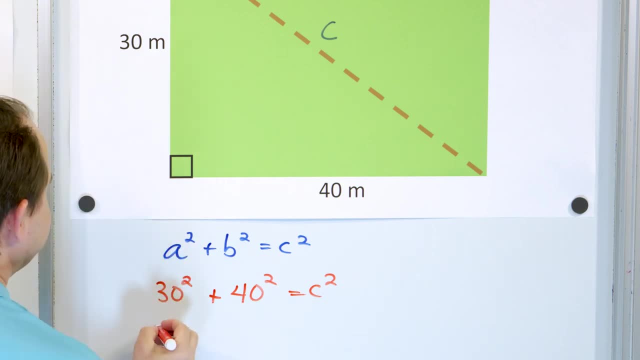 And that's going to equal c squared. All right, now you know that three times three is nine. So if three times three is nine, then 30 times 30 is going to be 900.. If you're not sure, dump it in. 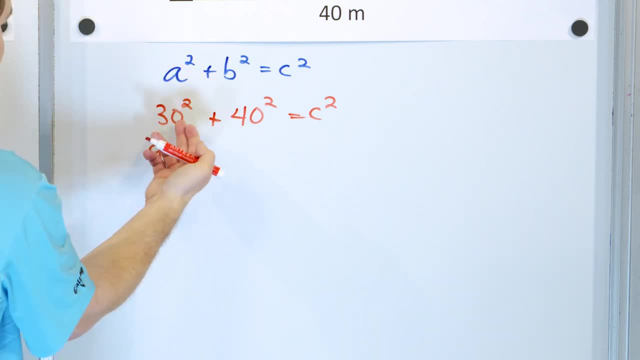 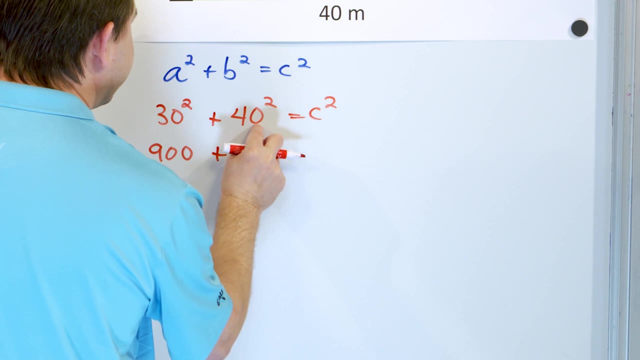 a calculator. But that's what you're doing. Three times three is nine And then, because you have the zero there, you're essentially adding two zeros because you're squaring, you know, two zeros there. same deal here: Four times four is 16.. But because we're squaring two zeros, we end up adding two. 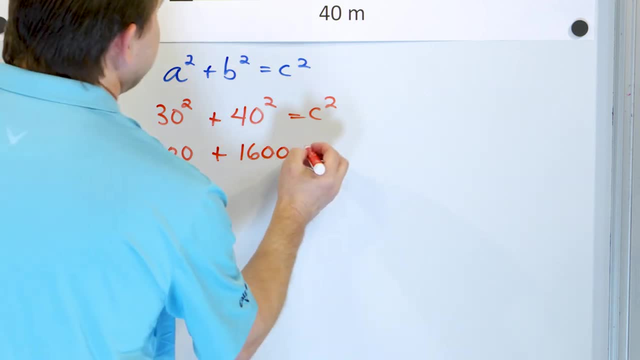 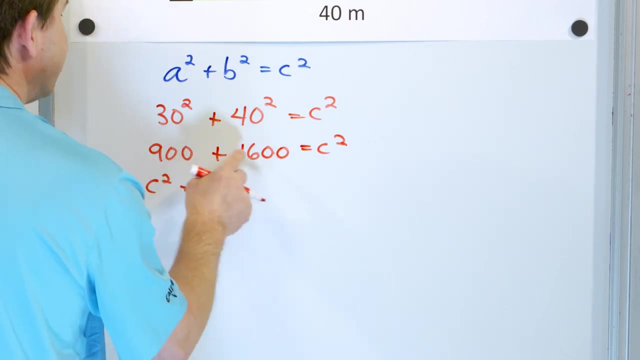 zeros on the end and it becomes 1600, 1600. And this is going to be c squared. So we'll flip it around And we'll say that c squared is 900 plus 1600.. Nine plus 16 is 25.. So 900 plus 1600 is. 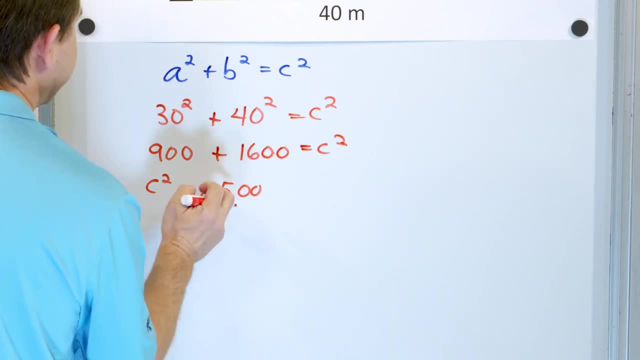 2500. And this is supposed to be an equal sign. So what we have? let me rewrite this: c squared is equal to 2500. And this is supposed to be an equal sign. So what we have, let me rewrite this: 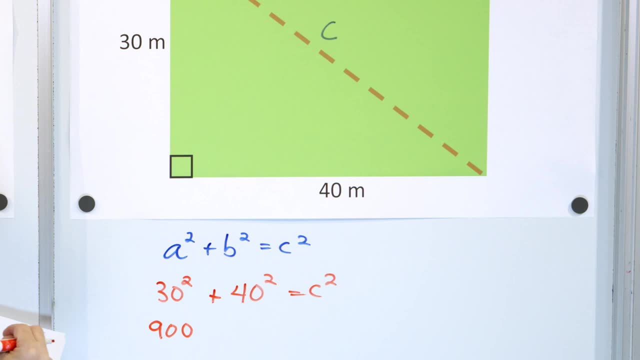 nine, then 30 times 30 is going to be 900.. If you're not sure, dump it in a calculator, But that's what you're doing. Three times three is nine, And then, because you have the zero there, you're essentially. 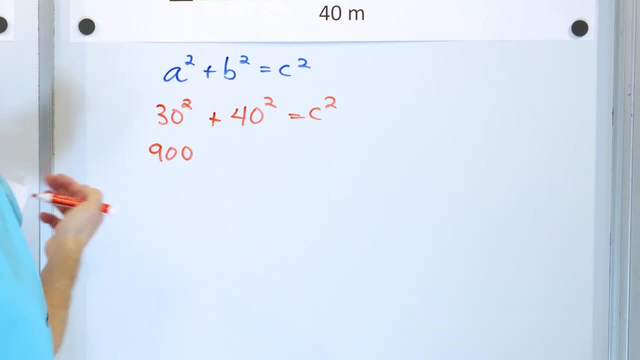 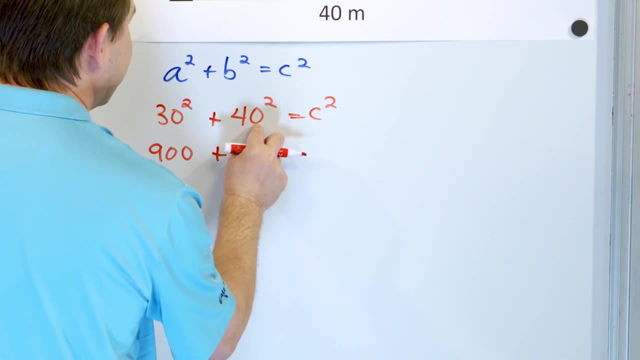 adding two zeros. because you're squaring, you know, two zeros. there is essentially 30 times 30 gives you 900.. Same deal here. four times four is 16.. But because we're squaring two zeros, we end up adding two zeros on the end and it becomes 1600, 1600. And this is going to be c. 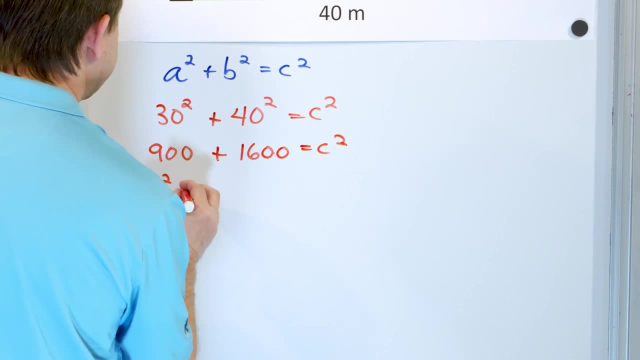 squared. So we'll flip it around And we'll say that c? squared is 900 plus 1600.. Nine plus 16 is 25.. So 900 plus 1600 is 2500.. And this is supposed to be an equal sign. 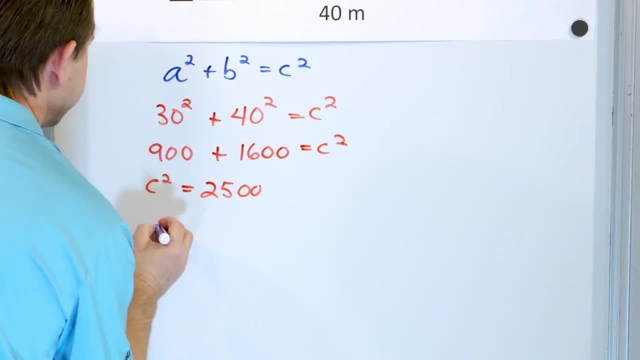 So what we have? let me rewrite this: c squared is equal to 2500.. We want to solve for c the length of the longest side of that triangle to get rid of the square. then we want to do the opposite, the square root, and we're going to have to do it to both sides to solve this equation. And when we 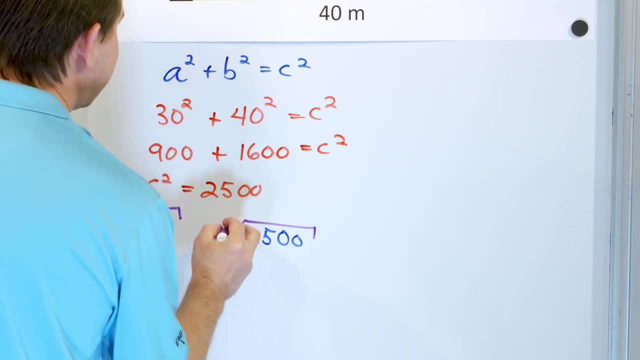 apply our own square root to solve something we have to add a plus or minus, Because this equation, c squared is equal to this. it really takes two solutions. If you think of a positive number, you're going to have to add a plus or minus. So we're going to have to add a plus or 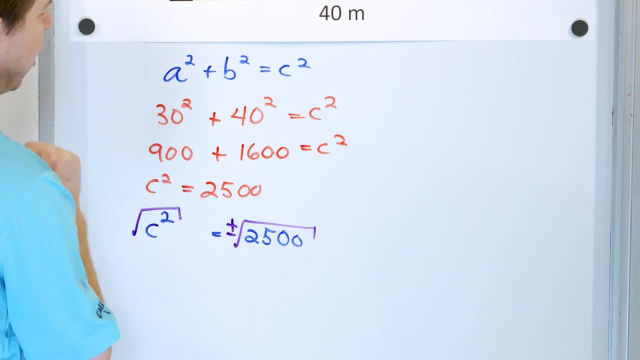 minus. So we're going to have to add a plus or minus. So we're going to have to add a plus or minus, And then we're going to have to add a negative number squared can give me 2500.. And a negative number squared can always also give me that same positive value. But we know in real life. 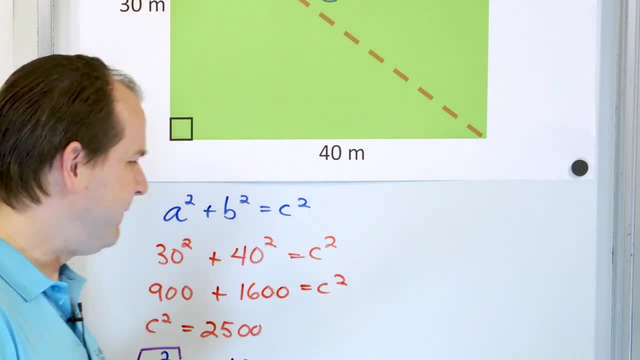 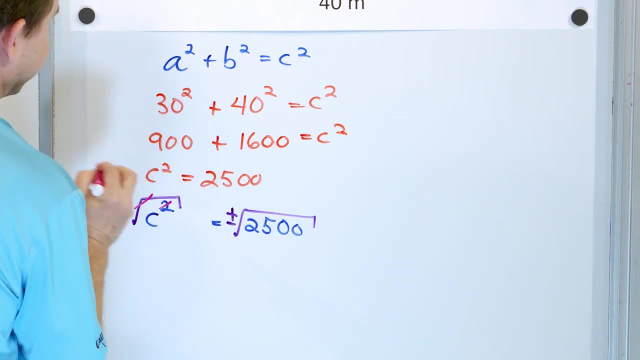 that we're going to discard any solution. that's negative because we can't have negative lengths of a fence. So we see over here that the square cancels with the square root and you're left with: c is equal to the plus or minus. the square root of 25 is five. So the square root of 2500 is: 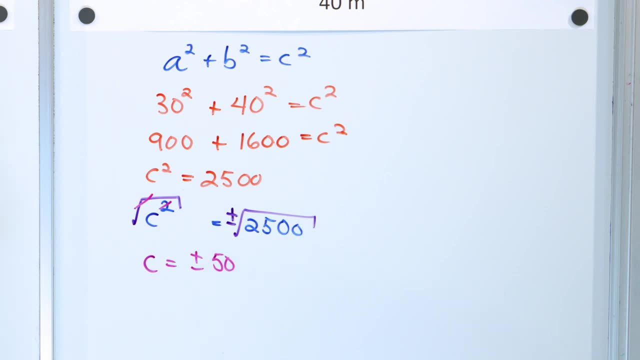 actually 50. If you're not sure about that, you can dump that in a calculator to verify or just go backwards. 50 times 50 gives you the 2,500. So we have a plus or minus 50.. As I said, 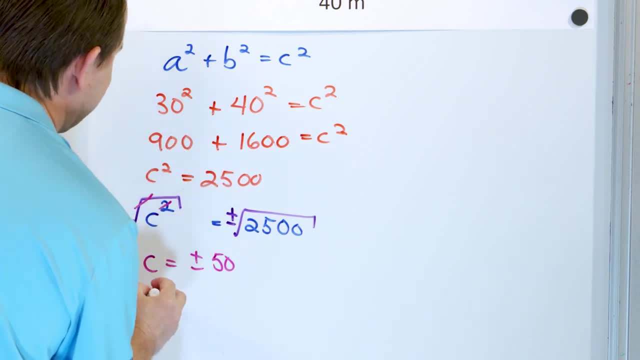 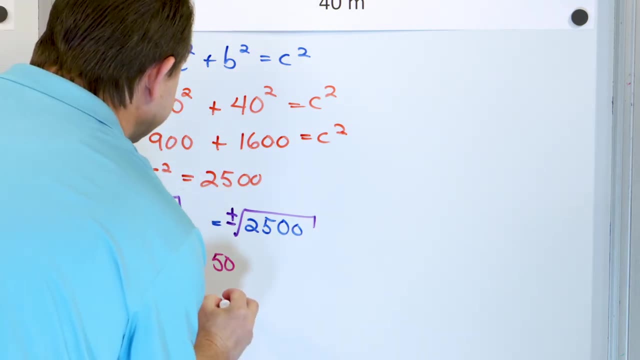 50 squared is this, and negative 50 squared is this as well. but we can't have negative lengths of the triangle. So the answer is positive, 50. And since all the units were in meters, the length is meter. Now, the length of this fence that we've calculated from corner to corner is: 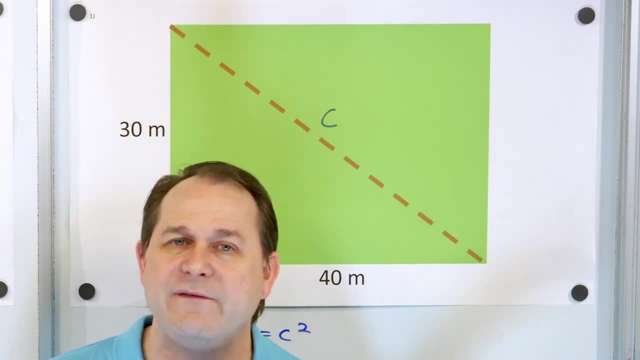 exactly 50 meters long. Now think about it. I told you in the previous lesson that there are a couple of triangles with special lengths that you can remember. 3,, 4, 5 is a triangle. that is always a right triangle: 3, a length of 3,, a length of 4, and the hypotenuse being 5.. So if 3,, 4,, 5 is a 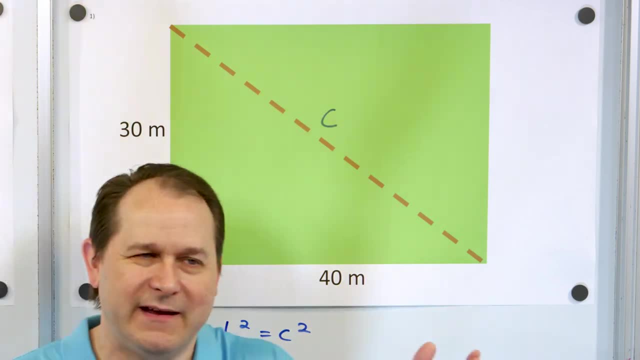 right triangle, then 30,, 40, and 50 is just kind of a larger version of that. So it's also a right triangle. So you could have predicted the answer if you thought about it ahead of time. but you know it's good to solve these things and learn. All right, let's take this one down, We'll do our. 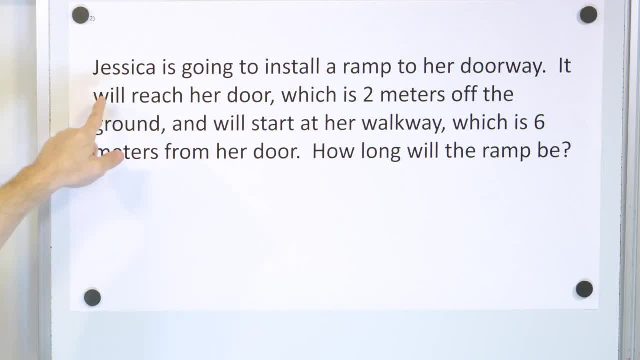 next problem. All right, Here's problem number two. Jessica is going to install a ramp to her doorway. It will reach her door, which is two meters off the ground, and will start at her walkway, which is six meters from her. 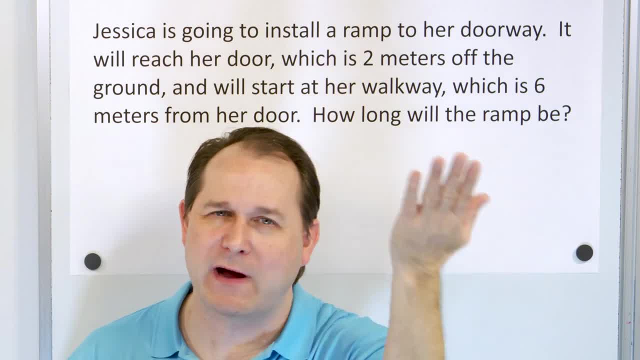 door. How long will the ramp be? So it's a ramp right. That means it's going to form a triangle, a right triangle. You're told how far away it is from the door. You're also told how tall, kind of. 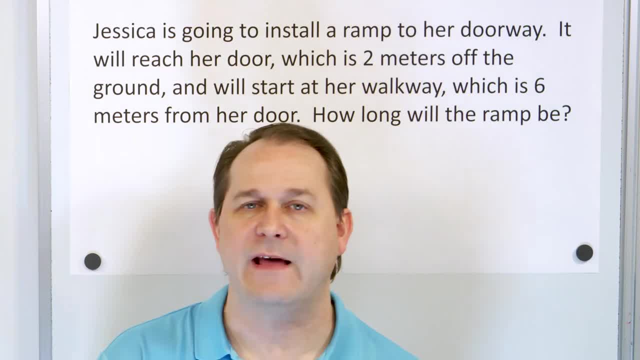 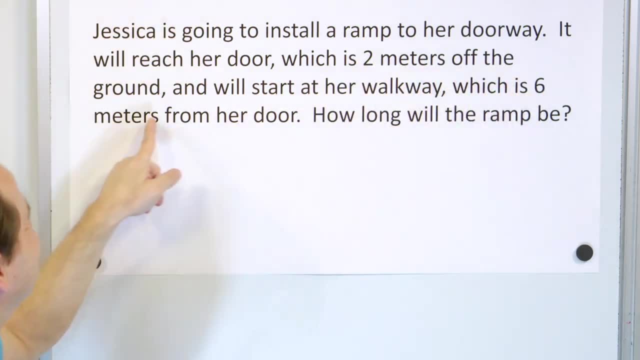 the bottom of the door step is, So you need a ramp that's going to fit into those dimensions. So let's draw a picture. The ramp of the door is two meters off the ground and we're starting the ramp six meters from the doorstep. 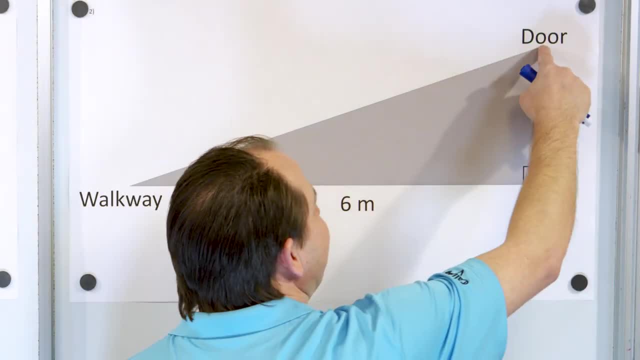 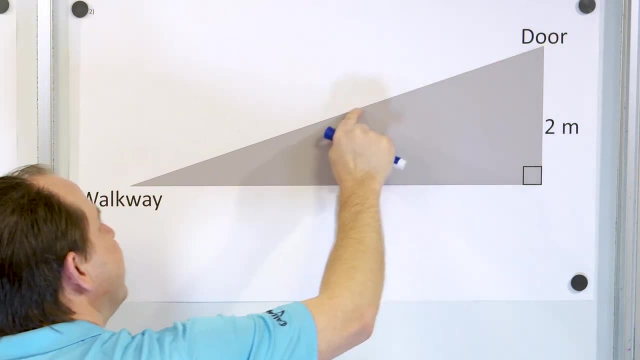 So we have a situation like this. So we have a door here that's elevated, it's two meters off the ground and we're going to start building this ramp six meters away from the door. So what we're trying to find is the distance of this slanted length, because it's asking us: how long will the 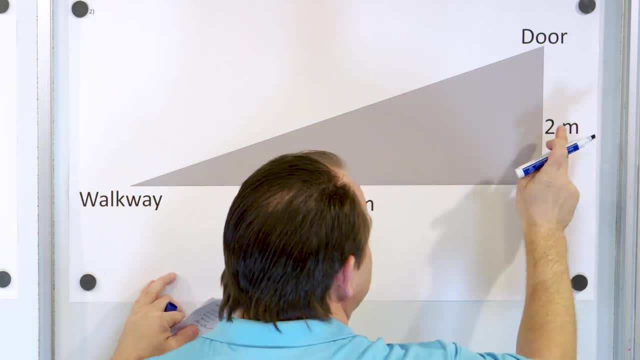 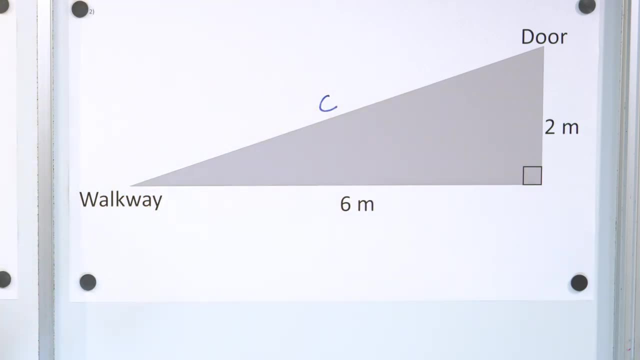 ramp be. So this is a right triangle: A and B or B and A, it doesn't matter there. But the longest side, the hypotenuse, opposite the 90 degree angles, we have to call that C there. So we know from the Pythagorean theorem: A squared plus B squared is C squared. So let's plug in what? 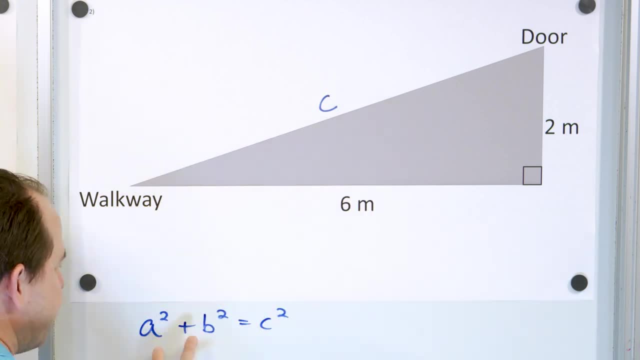 we know. We know one side is six, so that can go into A. It doesn't really matter, they're just added together. You could call this B if you want. it doesn't matter, We'll call it six squared B. 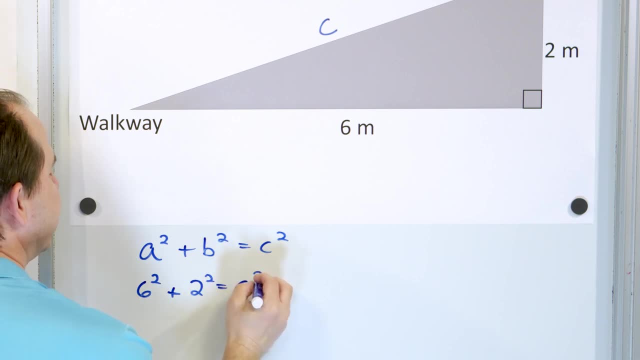 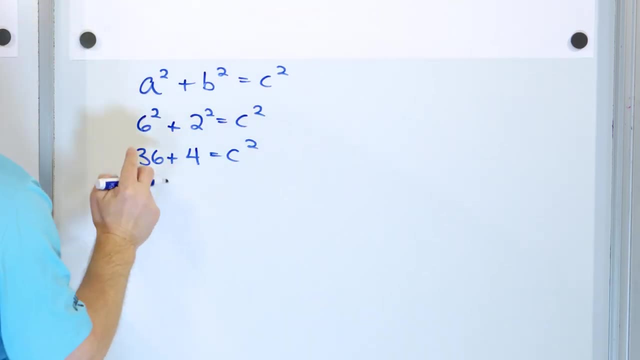 we're going to call two, So that's two squared and that's equal to C squared. So we have six times six, 36.. Two times two, four. Now let's flip it around. Let's put the C over on the left: 36 and 4 is 36.. 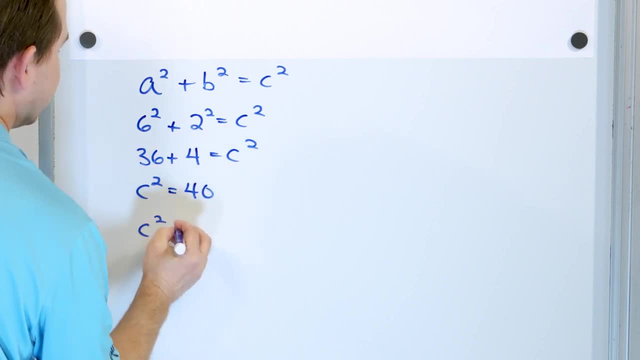 36 and 4 is 40.. So let me rewrite this: C squared is 40.. How do we get rid of that square? Well, we have to do the opposite of a squaring operation, which is a square root, If I do it on one side. 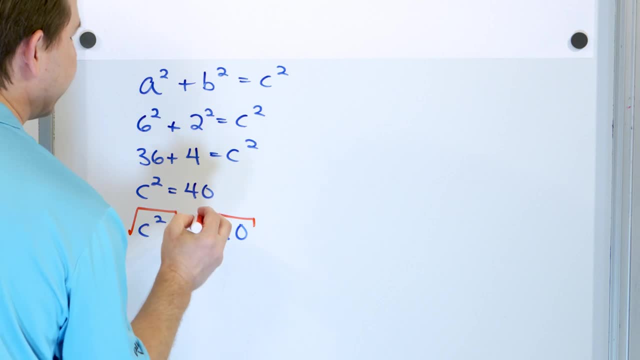 I have to do it on the other side And because I apply my own square root to solve the equation, I have to insert a plus or minus, because there really are two answers to this, one positive and one negative. But when we're talking about distances of a ramp, we don't really have a 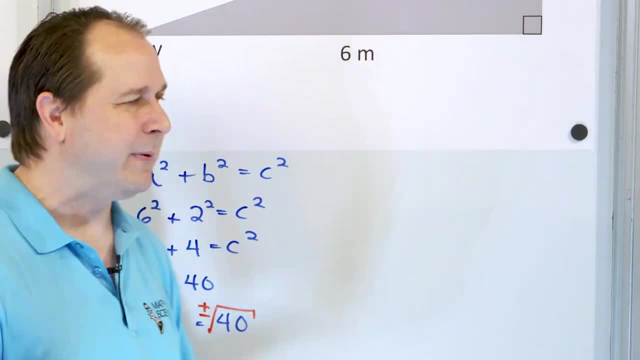 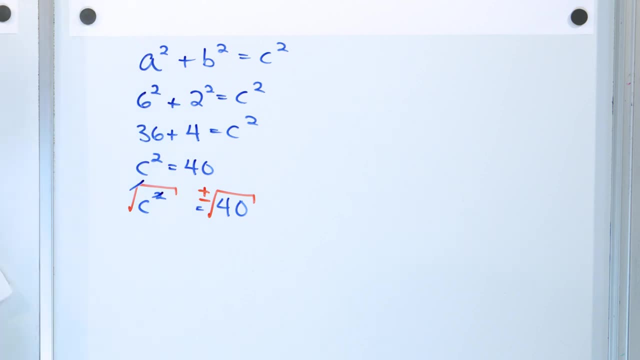 negative ramp distance. It's not physical, So we're going to throw that away, But just for fun we're going to go ahead and put the plus minus there, All right? So the square root cancels with the square, leaving behind only the distance C And it's going to be plus or minus the square. 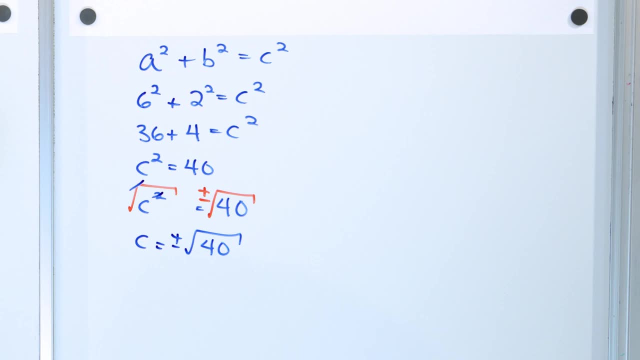 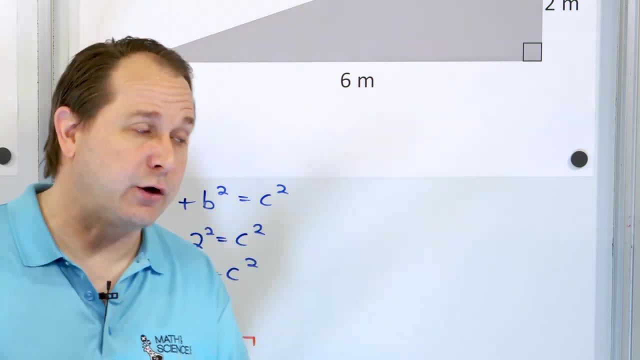 root of 40.. Now, what is the square root of 40?? I'm not a human calculator, so I cannot think of the of the decimal equivalent of that. I mean, I know 6 times 6 is 36.. That's not quite long enough, so. 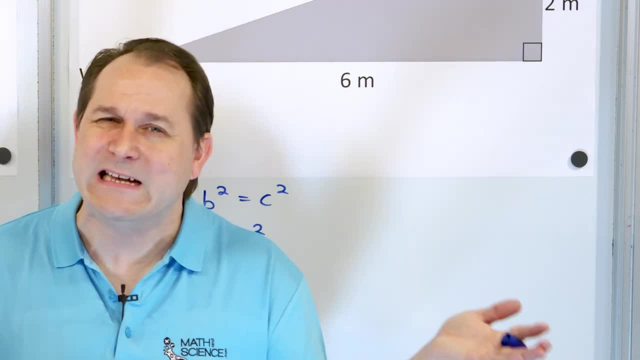 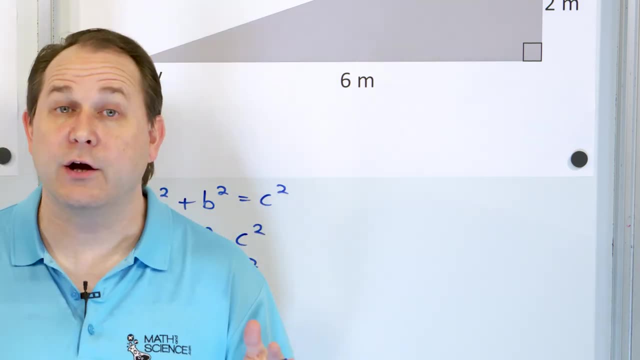 it's going to be a little more than 6.. I know 7 times 7 is 49, which is a little bit too big. So it has to be between 6 and 7. And I know that, But I don't know exactly. So let's go back and use. 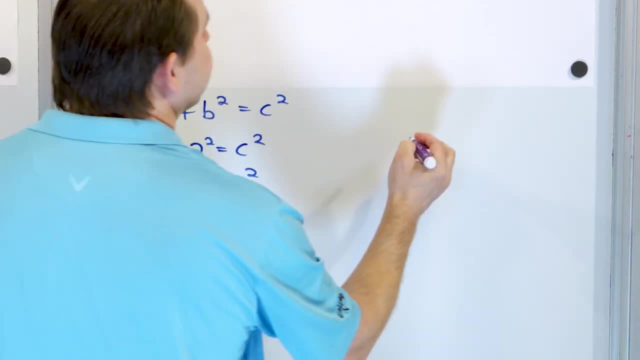 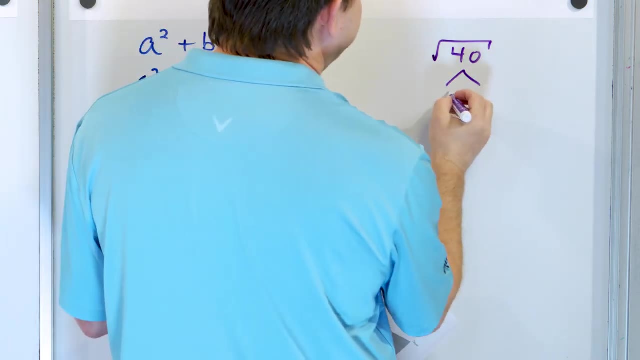 our skills from before. We're going to simplify this radical. We're going to put square root of 40 here. We're going to simplify it Now. I can do 10 times 4 or whatever I want. I'm going to do 8. 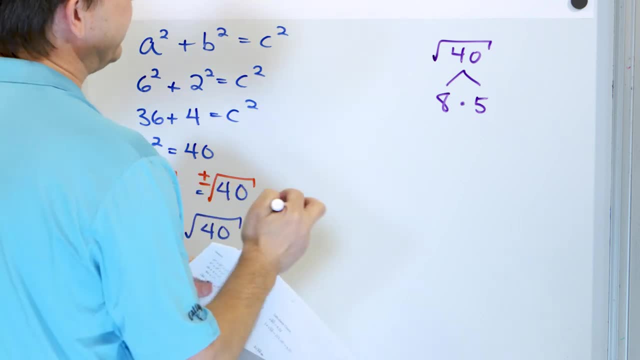 times 5, just because that's the first thing that comes into mind. But you can use anything you wish. The 8 you can write is 2 times 4.. And the 4 you can write is 2 times 2.. Now we're looking for pairs. 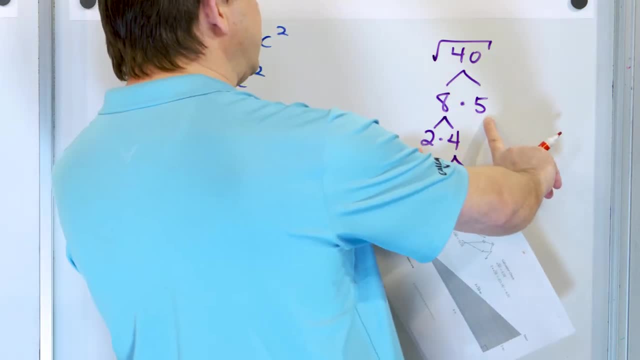 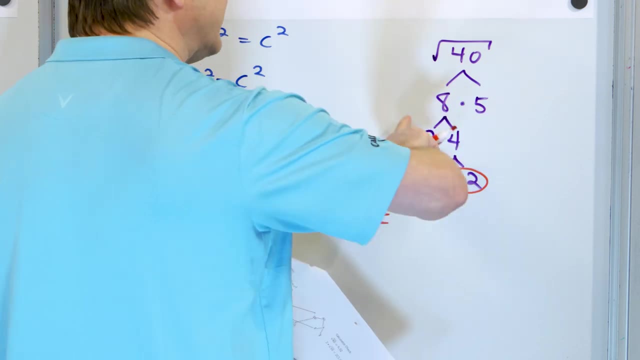 You see a pair of 2s here, because it's a square root Now the 2 and the 5, they don't have any partner pairs. So what's really going to happen here is the 2 is going to stay under, The 5 is. 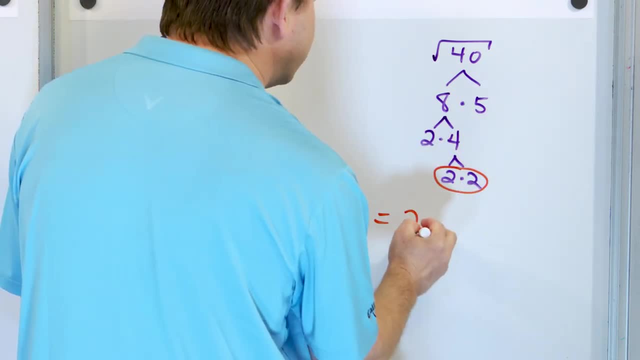 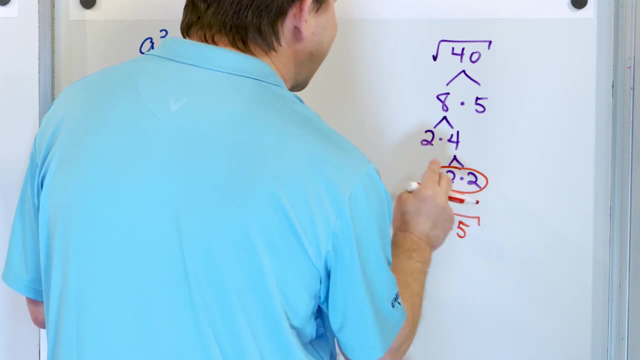 going to stay under, But this as a pair is a single. 2 is going to come out And underneath is going to remain the numbers that we have left behind: the 2 and the 5. But they're multiplied together because everything in this tree is multiplied together, And so, really, what you have, 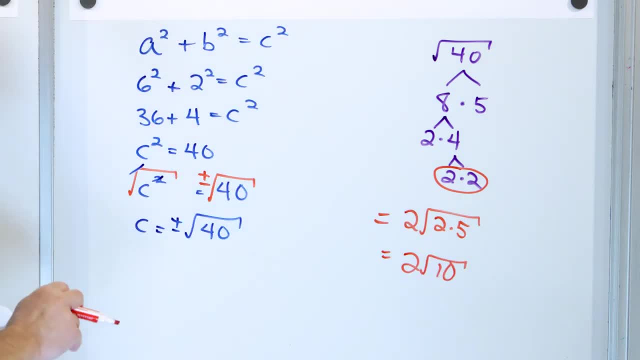 is 2 times the square root of 10.. 2 times the square root of 10.. And we said that the answer was plus or minus square root of 40, which is 2 times the square root of 10.. But we're throwing away the negative answer, So we're just going to put that c is equal. 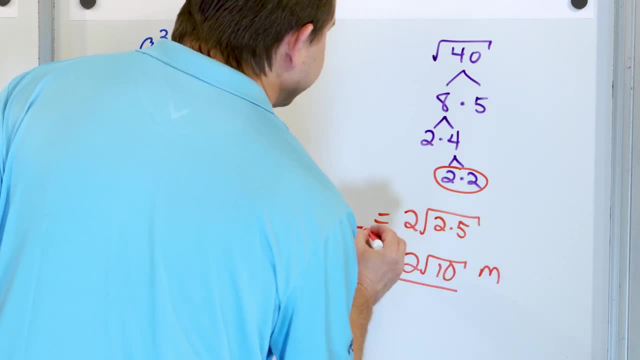 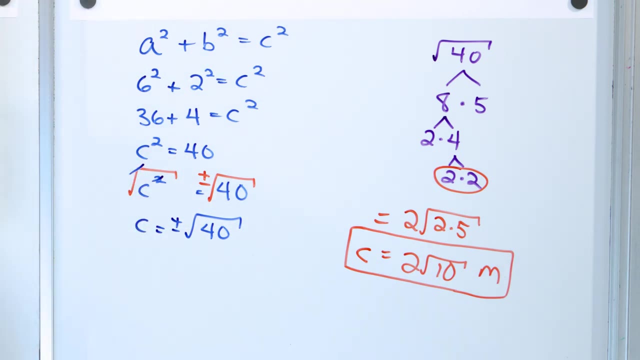 to 2 times the square root of 10.. And the unit is meters, because we were talking about meters throughout the entire problem. Now, since this is a wacky looking radical like this, if you were to dump this in your calculator, you would find out. 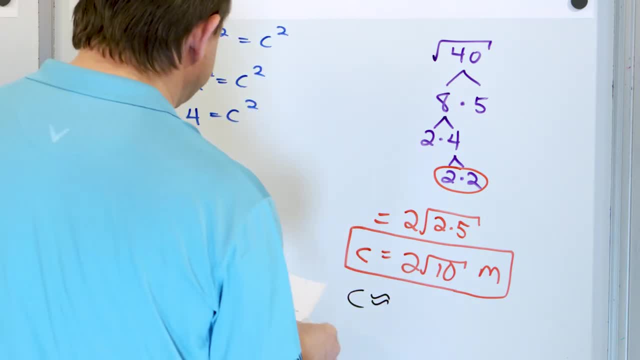 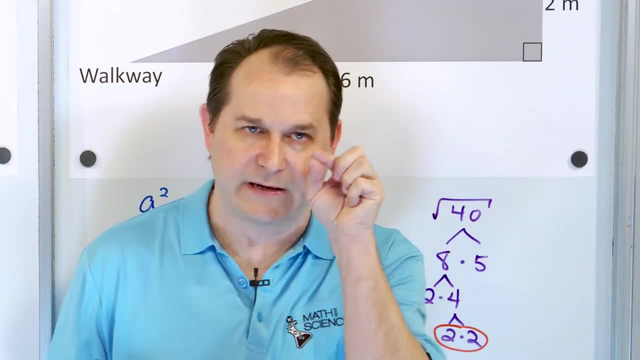 if you were to put in square root of 40 in your calculator, you would find out that it's approximately 6.32.. Now, these radicals like this. when you dump them in and you calculate them, you'll see that they go on forever. They're what we call remember irrational. Irrational means. 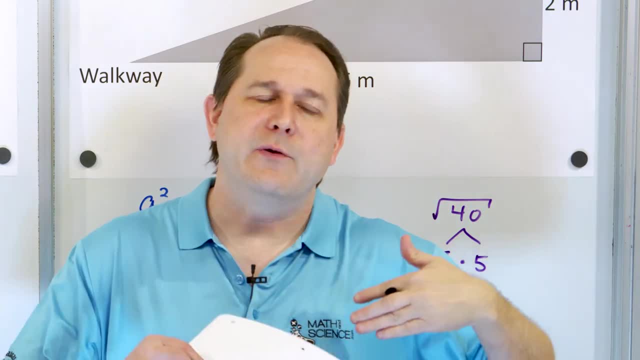 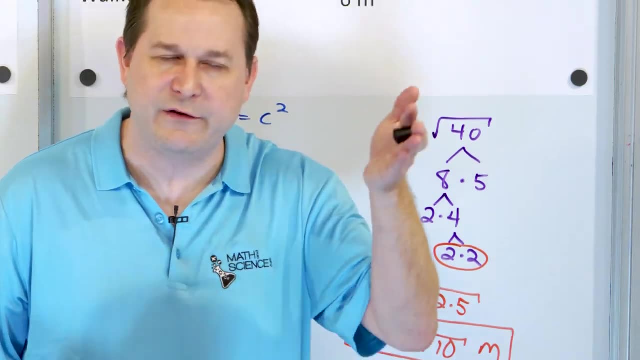 the numbers, the decimals go on forever and they never stop. So you'll have to round it. So this is an approximation. If you put square root of 40 in the calculator and execute and enter it, you'll get 6.32 with a bunch of decimals after it. So this is the rounded 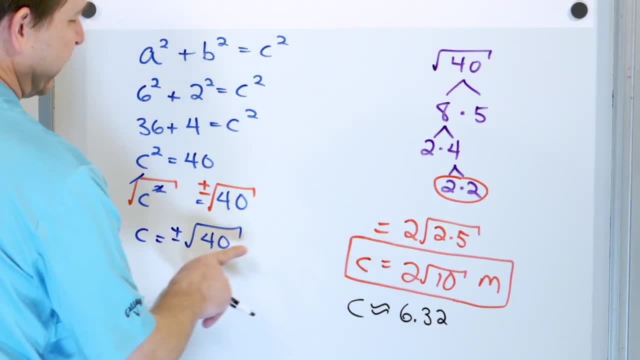 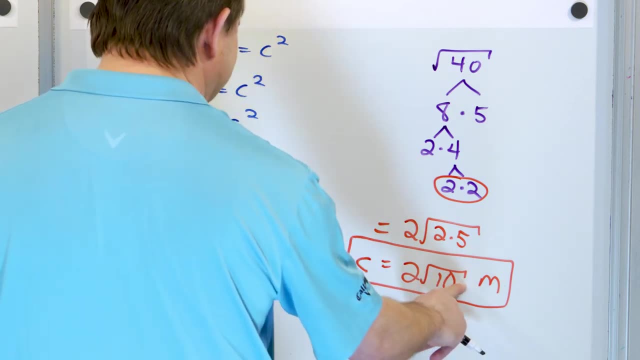 approximate value. What we calculated is our simplified version of this: 2 times the square root of 10.. If you put the square root of 10 into a calculator, you're going to get approximately 3.16.. And then, when you multiply by 2, this is what you're going. 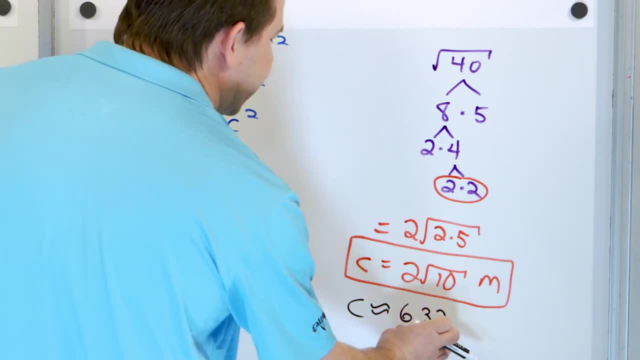 to get. So I guess what I'm trying to tell you. if you dump this in your calculator, you're going to get this. If you find the square root of 10 and then multiply it by 2,, you're going to get the. 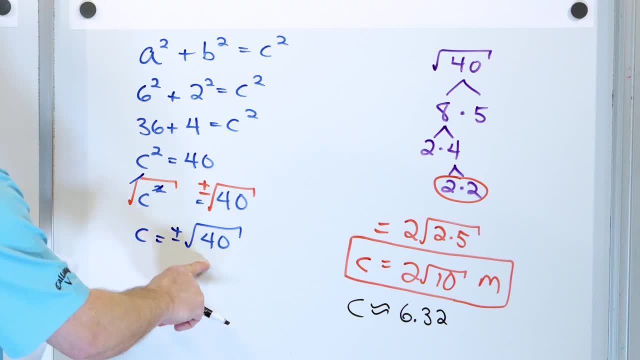 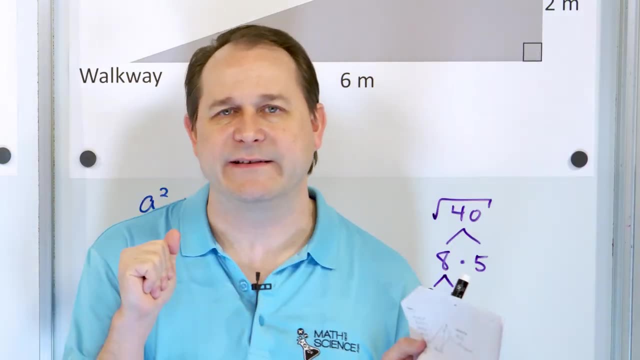 same answer. So this is just a simplified version of this, which again is approximately 6.32 meters. And remember we said it has to be between 6 and 7, because 6 times 6 is 36.. 7 times 7 is 49.. 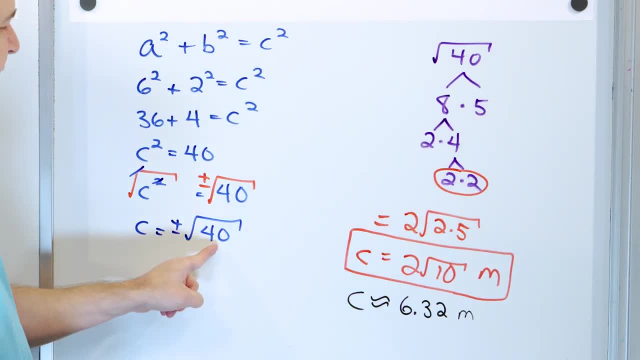 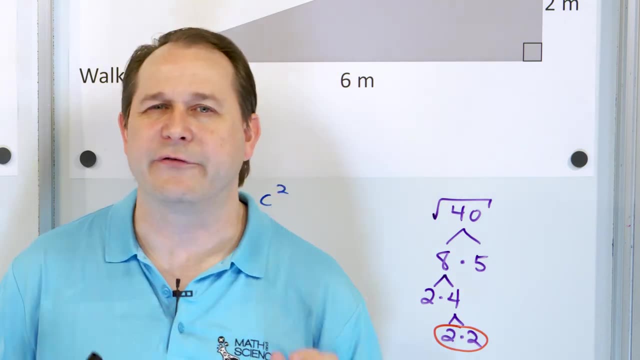 And we were shooting for 40,, which is between 36 and 49.. So the answer is, as we said, 6.32,, which is in that range somewhere. We're not human calculators, So if you get a radical that you 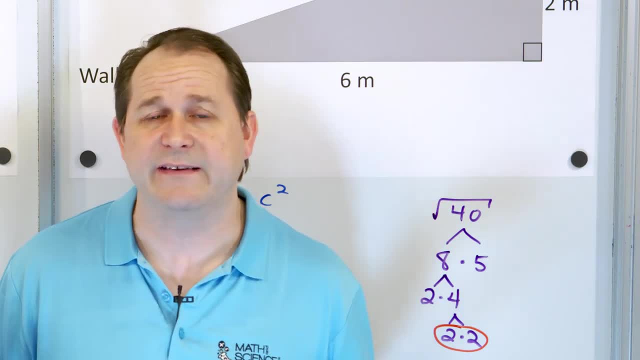 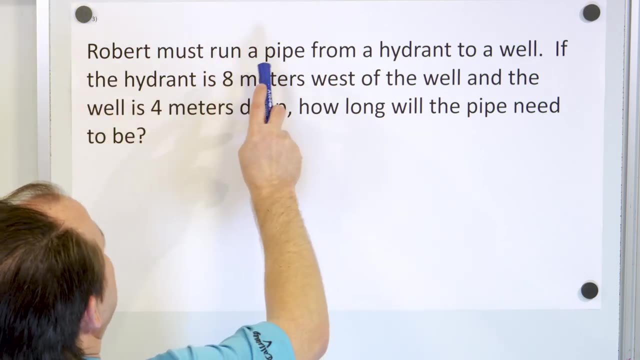 don't know the answer, to just simplify it as much as you can And you circle it and say this is the exact answer. All right, let me take this down, We'll do our next problem. All right? Our next problem: Robert must run a pipe from a hydrant to a well If the hydrant is eight meters wet. 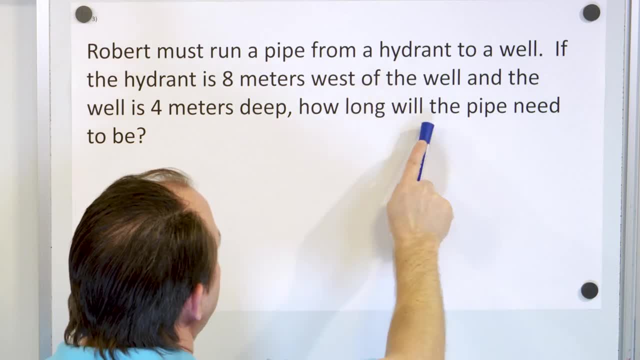 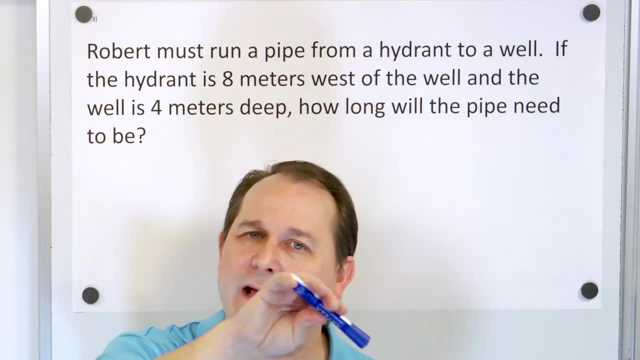 of the well, and the well is four meters deep. How long will the pipe need to be? So it's kind of an upside down triangle. We're trying to lay a pipe which is gonna go underground at some angle. We know how far away from the well it needs to be. 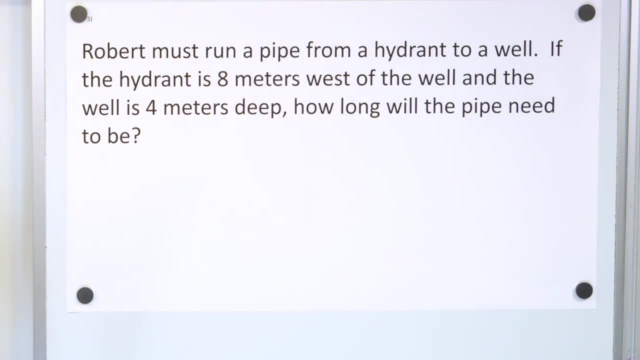 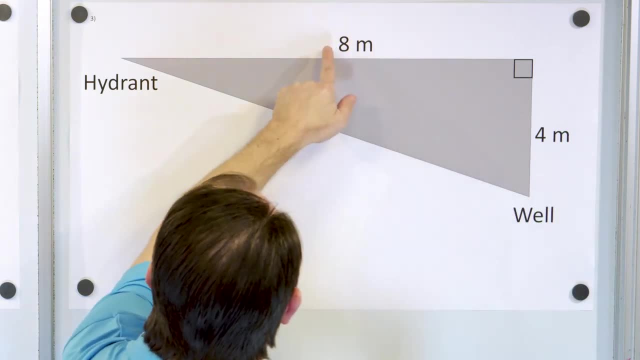 how far west and we know how deep the well is. So let's draw a picture. So here we have some sort of hydrant, here we have some well. right, There's some vertical distance in the well where this hydrant a source of water or whatever it is. 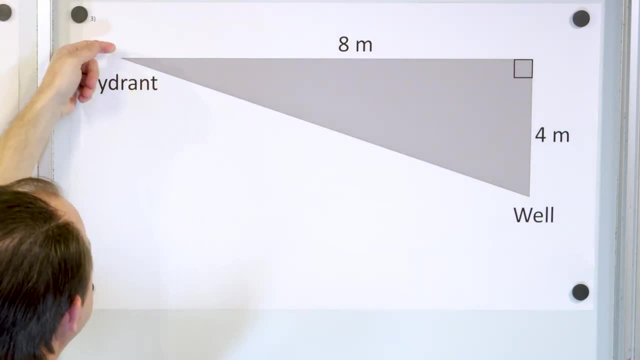 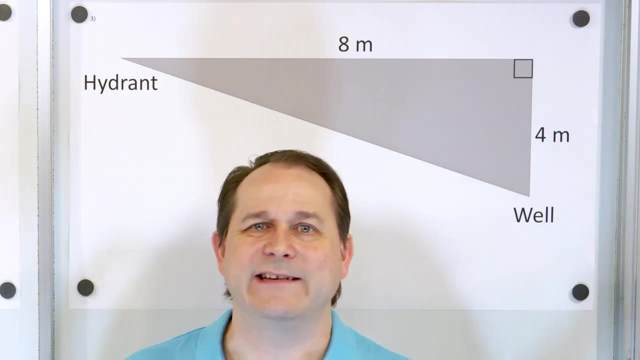 a pump is this many meters- eight meters west of this location. So if you're gonna run a pipe from here to here, how long does this pipe need to be? It would be completely wasteful to just like guess and say, well, give me some pipe. 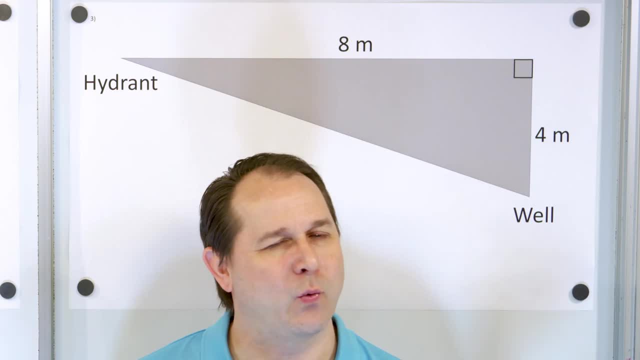 Let's see how long. let's just guess and we have extra. That's not gonna work in the real world. You have to know how long and how much you need. Maybe you add five or 10% as just extra, So you have a little extra, but you never wanna guess. 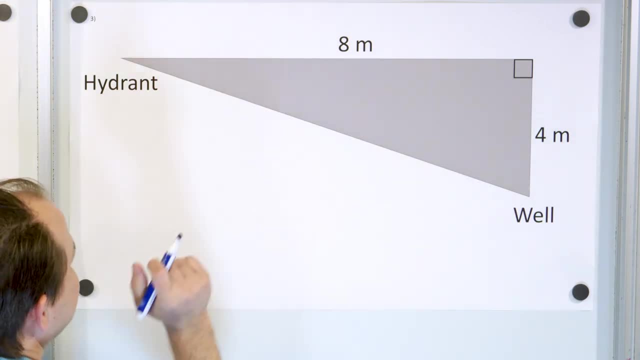 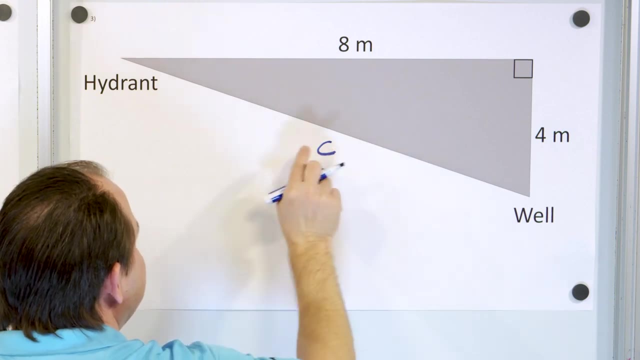 We have to calculate, So let's go and do that. This is an upside down triangle. We're gonna say this is A and this is B. The hypotenuse opposite is always opposite of the right angle, the longest side, That's what we call C. 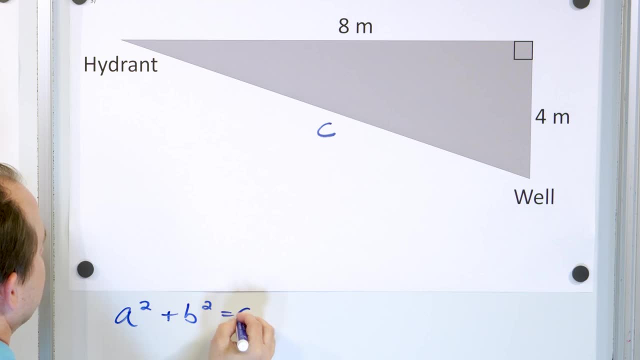 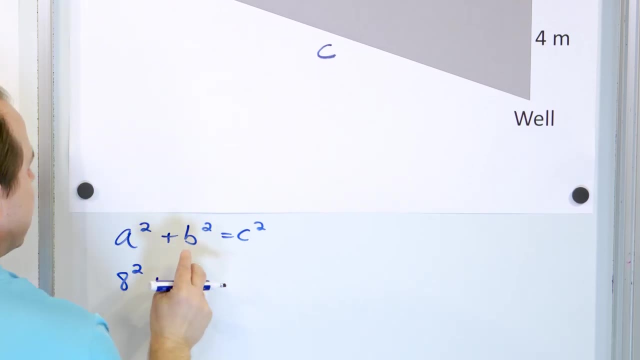 So we say A squared plus B squared equals C squared. Now it doesn't matter which one you call A and B. Let's call eight A, so that's squared B. we're calling four, so that's also squared. And then we have C squared. 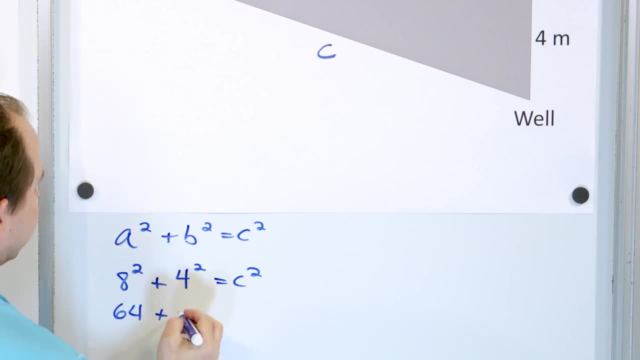 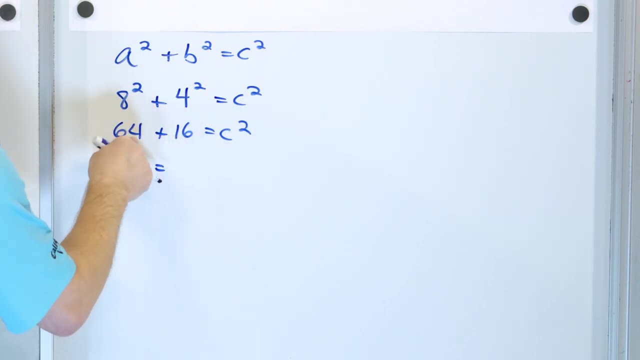 Now we know that eight times eight is 64.. We know four times four is 16.. Let me flip it around. put C squared on the left, So when you add this, you'll get, with the six, 70, and the 10 is 80.. 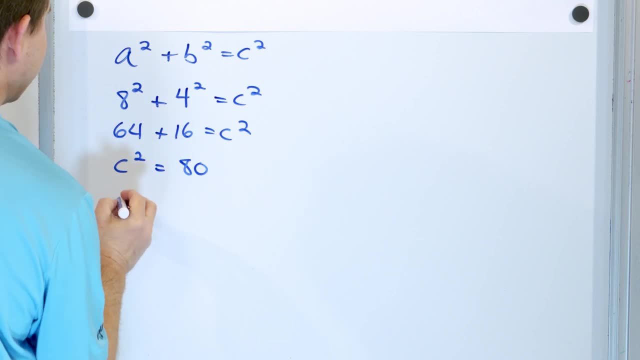 So you're gonna get 80 right here. So what we need to do is take the square root of both sides of this thing to actually calculate the answer. Because we have C squared. we wanna get rid of the square root by using a square root. 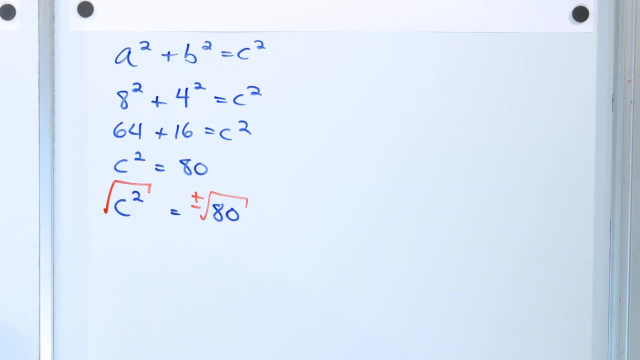 When we do that ourself, we have to add a plus or minus, Now the square, and the square root is gonna cancel, so we're gonna be left with the variable C and we have to figure out what is the square root of 80?. 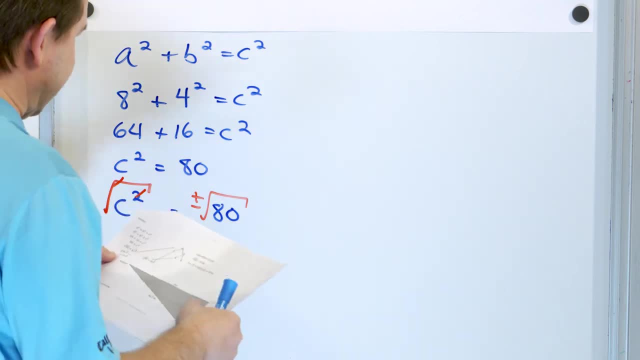 So we're gonna have to figure out what is the square root of 80? Now again, I'm not a human calculator. I don't know what that is right, But I know that 10 times 10 is 100.. 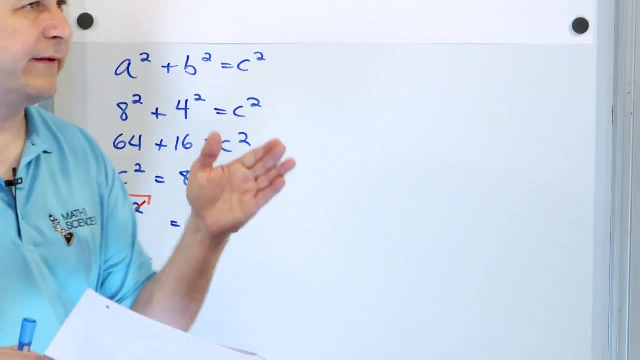 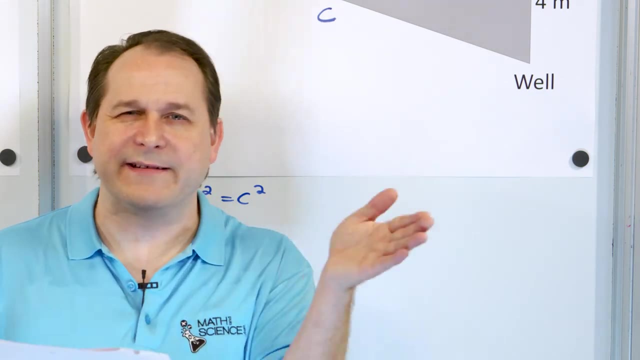 I know that nine times nine is 81, but I want the square root of 80.. So it's gonna be a little less than nine, because nine times nine is 81.. Eight times eight is 64.. So I know it's gotta be somewhere between eight and nine. 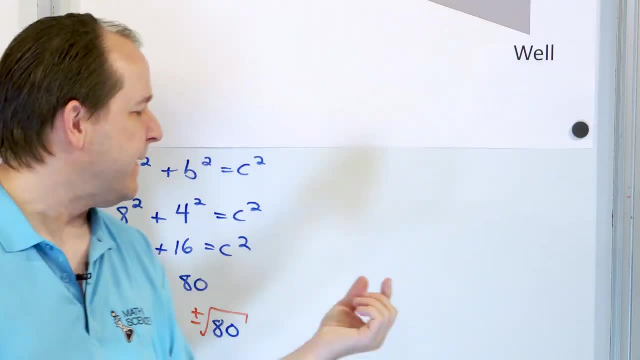 because eight times eight is 64, and nine times nine is 81.. And we're trying to find the square root of 80, which is in that range. So I know it has to be pretty close to nine actually, but definitely between eight and nine. 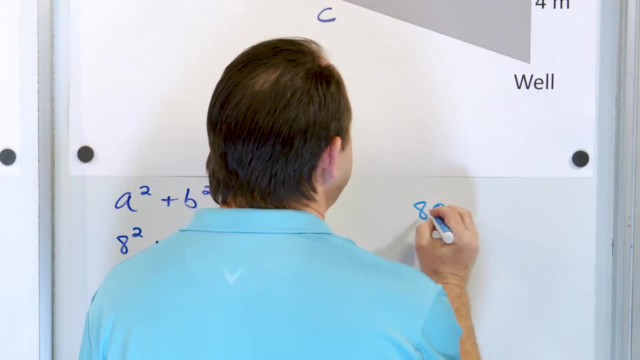 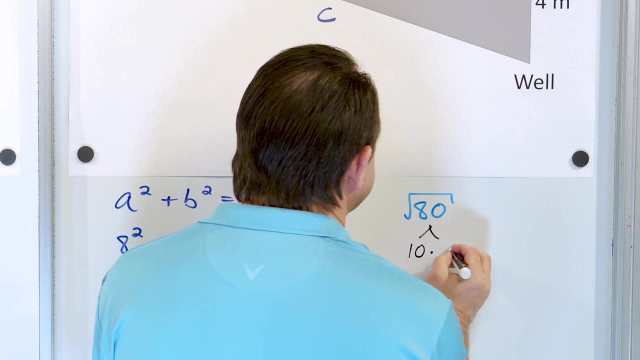 but definitely between eight and nine. So let's figure out how to simplify the square root of 80.. Now you can do anything you wish here. Okay, I'm gonna say 10 times eight. If you know something else, like 40 times two, for instance, that's fine too. 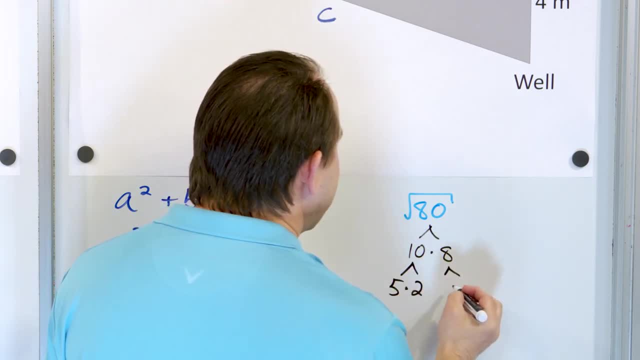 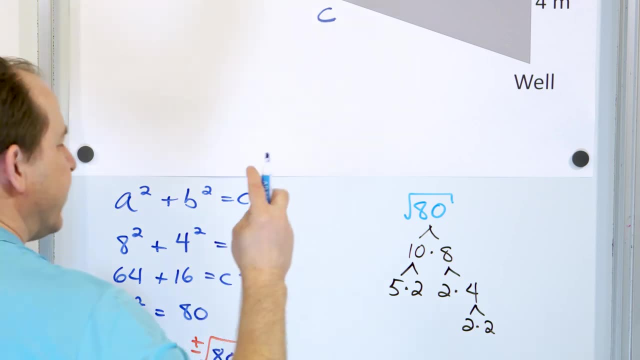 All right. so here I'm gonna do five times two is 10, and here I'm gonna do two times four is eight and four I'm gonna do two times two. All right, So I'm looking for pairs. 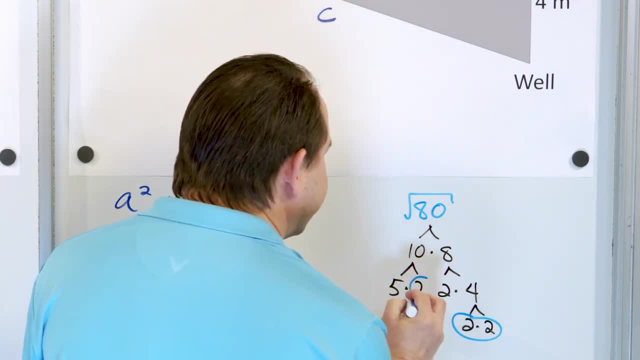 Here's a pair of twos and here's another pair of twos. I'm allowed to circle one and two. Well, these, they're still at the bottom of the tree and this five, unfortunately, doesn't have any partner. 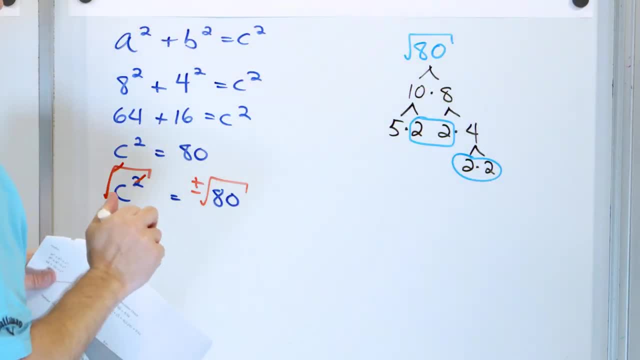 This four doesn't count. He's not in the bottom of the tree. Remember, we're doing this only with things in the bottom of the tree. So what you're gonna have is this: two is gonna come out because a pair pairs come out. 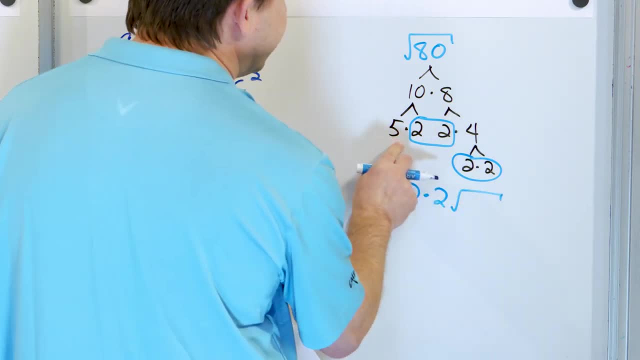 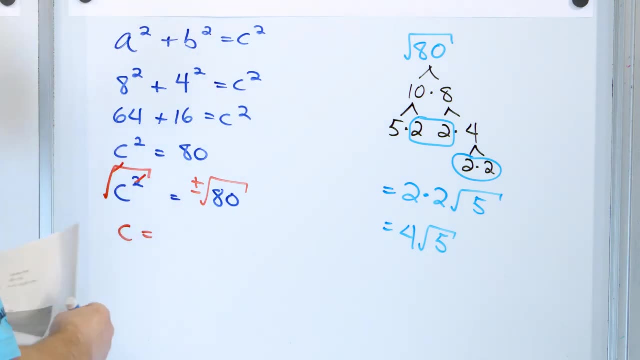 This two is gonna come out. They're multiplied together and what's left over is underneath the radical, And so, since they're multiplied, here you have four, and then you have the square root of five, Four times the square root of five. 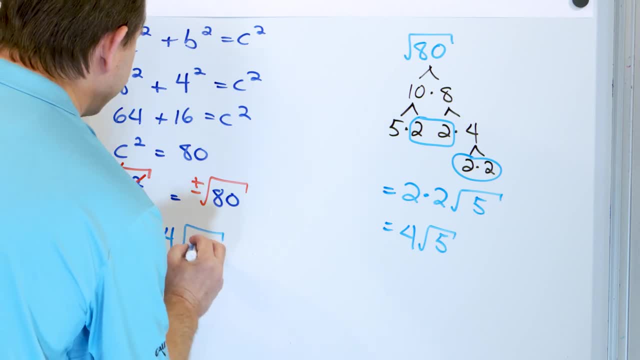 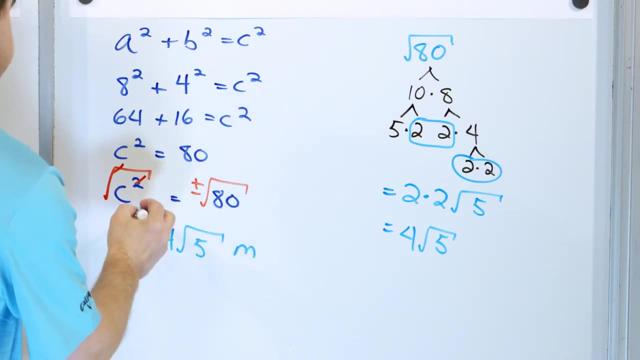 and that's what the value of C is: four Times the square root of five. And what unit are we dealing with? It's all meters in my problem, So that's meters. Now, this is the exact answer, right, Because this radical is exact. 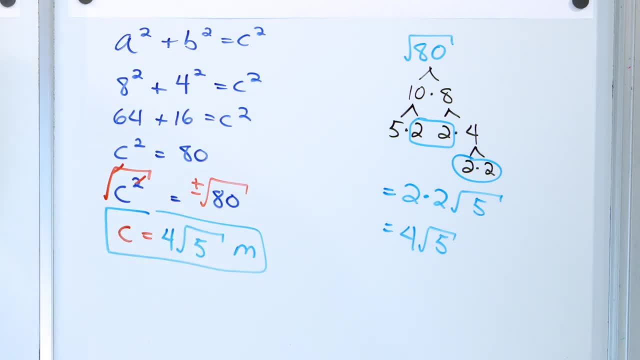 Remember this radical. if you calculate it, it goes on and on forever. If you dump this into a calculator, right, You will figure out that the answer you actually get is 8.94.. Now, of course, you have to round it. 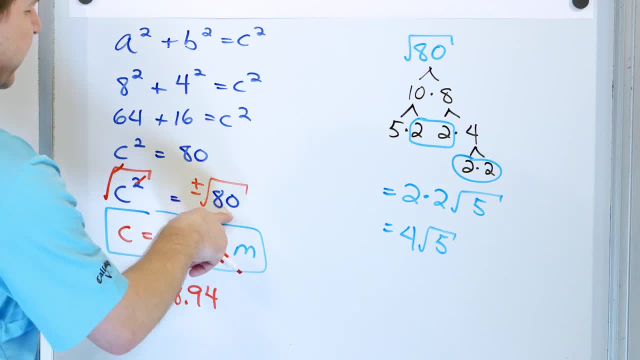 because the decimals go on forever. But if you put 80 into a calculator and actually take the square root, it's gonna be 8.94.. That makes sense because nine times nine is 81.. So that's really close. 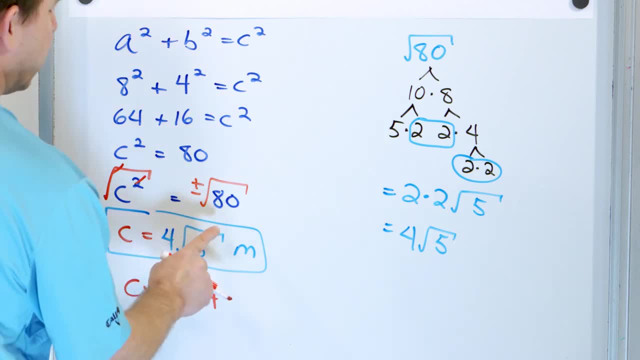 So it's just a little bit less than nine. all right, If you were to take square root of five and get that answer, you'll get 2.24 after you round it, And 2.24 times four if you carry enough decimals. 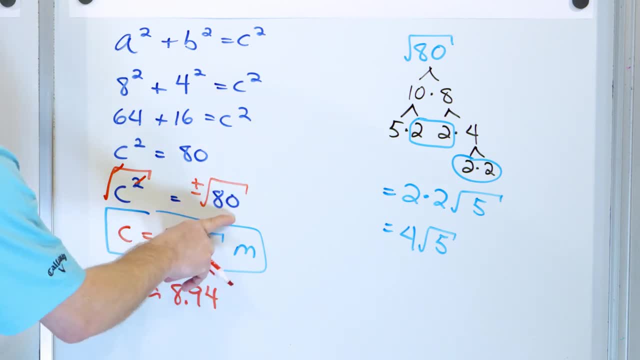 it's gonna be basically the same exact number. So the square root of 80 and four times the square root of five are exactly the same thing, which approximate. that's why I have the squiggly equal signs approximately equal to 8.94.. 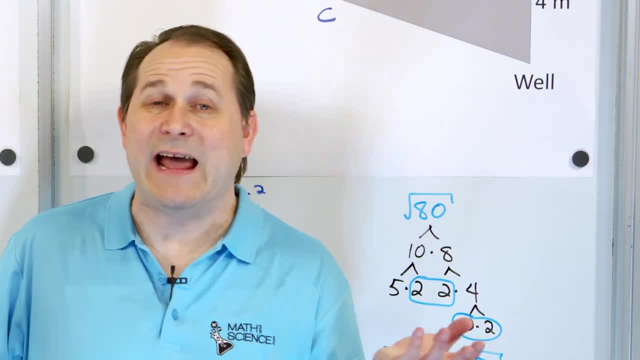 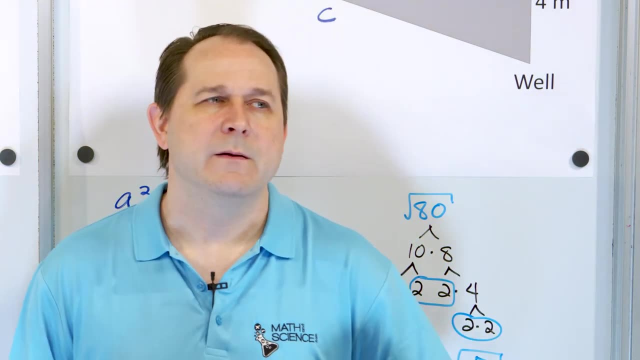 So if you're really doing this in real life and you calculate you need 8.94 meters, maybe you should buy nine meters, or maybe nine and a half meters of pipe, just so you don't mess something up. you have enough. 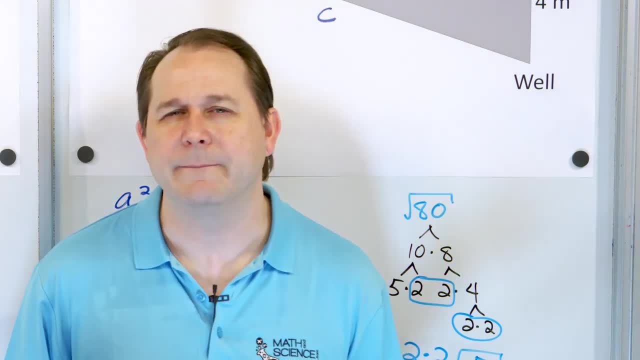 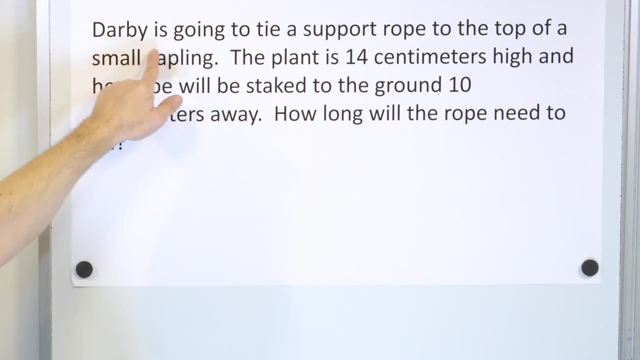 But you wouldn't wanna buy like 15 meters of pipe. that would be completely wasteful, right? So let's take this down and solve our last problem. All right, here's our last problem. Darby is going to tie a support rope. 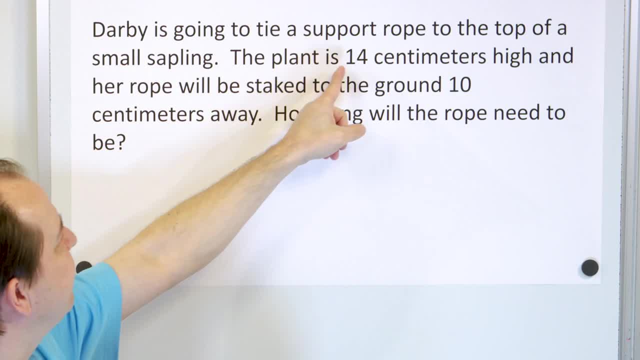 to the top of a small sapling. The plant is 14 centimeters high and her rope will be staked to the ground 10 centimeters away. How long will the rope need to be? So we're forming a triangle. we're staking a tree. 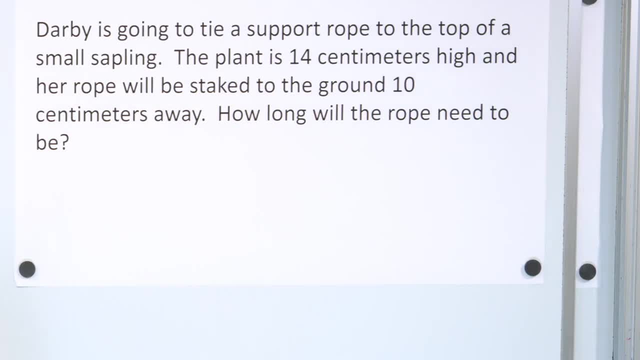 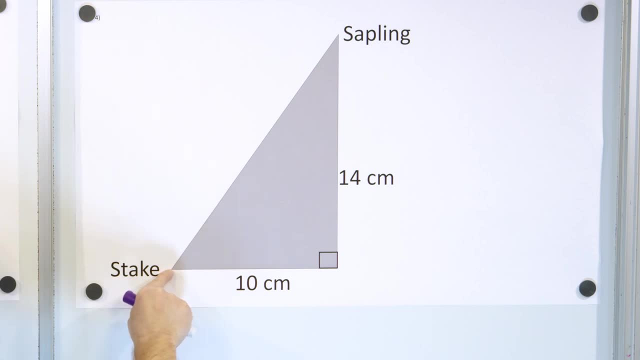 so it's gonna form kind of a triangle, coming off the top of that tree, the sapling, and it'll look something like this: So you have this tree which is this top of the tree, and we're going to stake the rope into the ground. 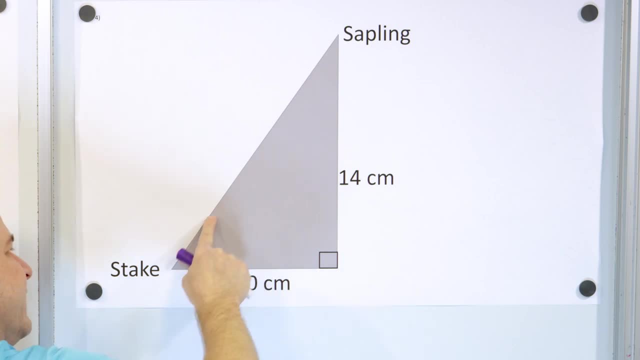 10 centimeters away and the tree is 14 centimeters tall. so the question is: how long does this rope need to be? We're gonna label that C because it's the longest side and it's opposite the 90 degree angle. 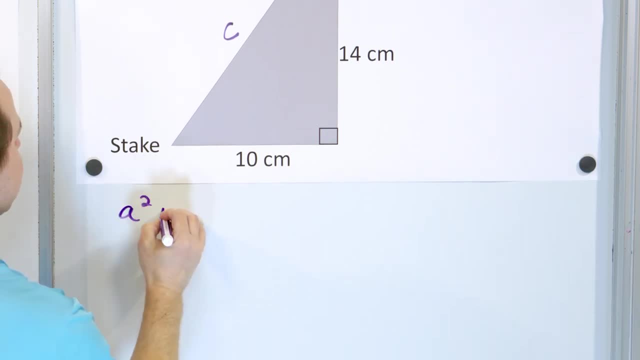 Since it's a right triangle, we know that A squared plus B squared is C squared. It doesn't matter which one you call A and B. so I'm gonna put 10 in here. 10 squared B is 14, so that's squared. 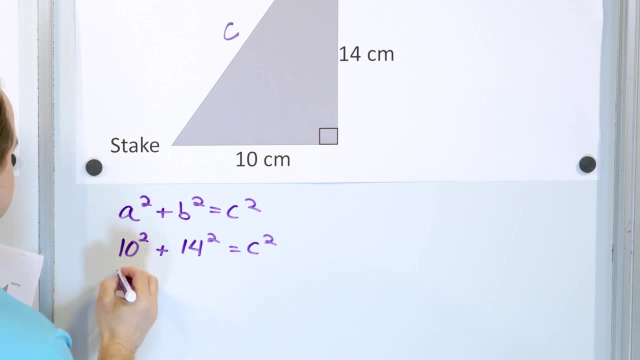 and then you're gonna have C squared. Now, 10 times 10 is actually 100, and 14 squared is actually 14 times 14,, 196, and that's C squared. When you flip it around, say, C squared is equal to. 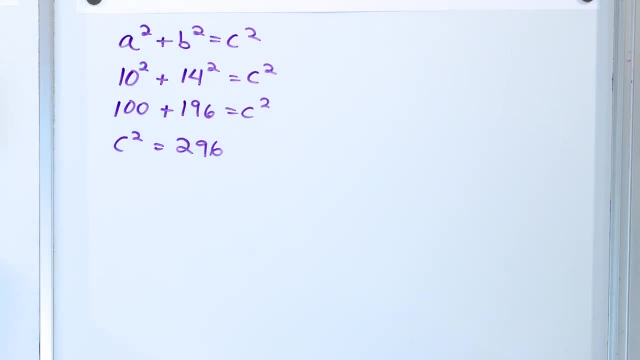 when you add these together, you get 296, right? So once we take the square root of both sides of this, on the left, all I'm gonna be left with is C, and on the right-hand side, it's gonna be square root of 296.. 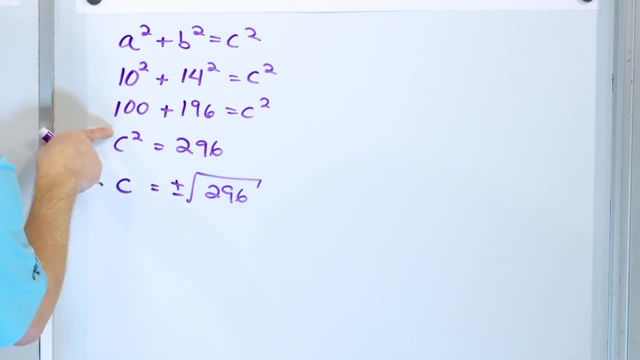 Make sure you understand what I did. I just took the square root of both sides. Square root on this side just gives me a C once they cancel. Square root on the right side is what I've written here and I have to insert my own plus or minus there. 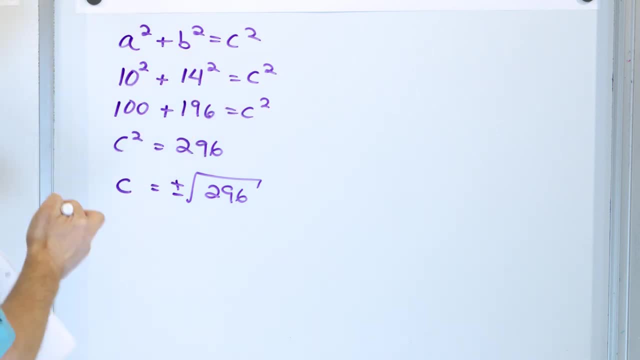 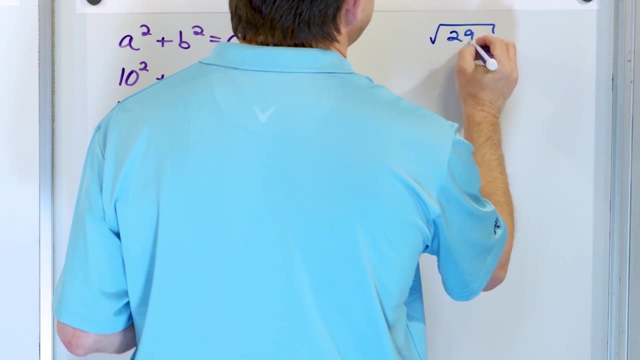 because I put my own radical in place. all right, Now I don't know off the top of my head what the square root of 296 is, so let's just simplify it as much as we can. 296.. Now, this is an even number, so I know it's divisible by two. 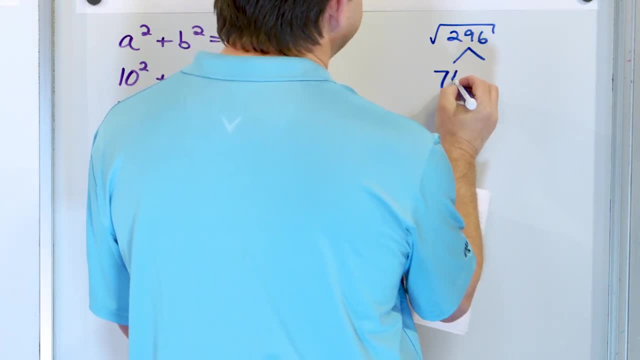 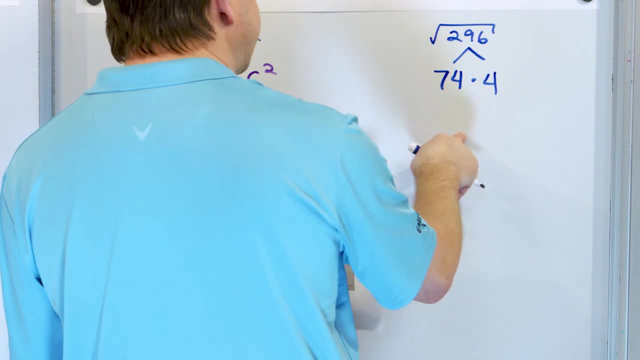 but once I play around with it a little bit, I realize it's also: divisible by four Turns out 74 times four is actually exactly equal to 296.. Now, this is an even number. You could split it apart, but it's only gonna be two times 37,. 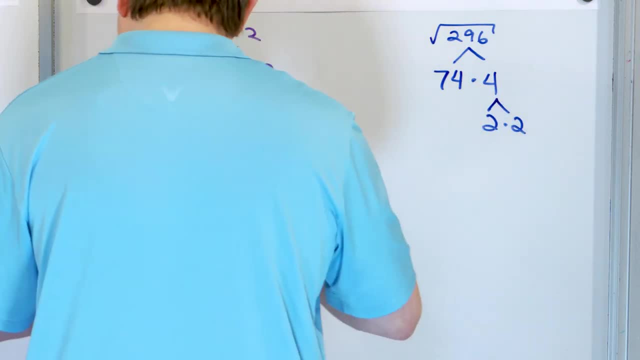 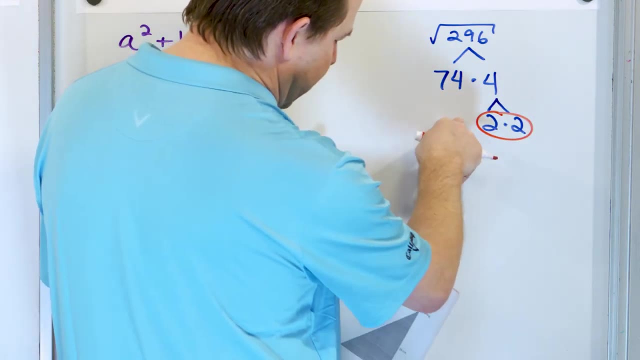 which isn't not gonna help me, because here I have a two times two and I'm looking for pairs, So here I have two times two, so I know that's gonna come out. This I could do two times, which is 37, but again I can't break 37 apart anymore. 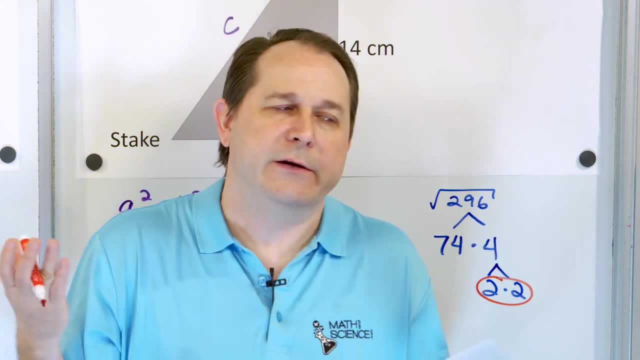 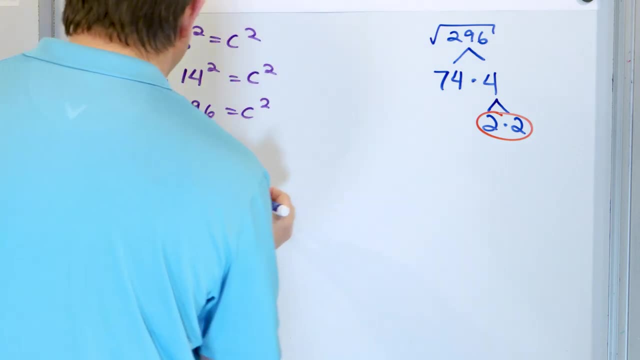 and I won't have any more pairs, so I might as well not even do it. You could if you want, but it's just gonna stay under the radical anyway. So what I'm gonna have at the end of the day is this: single two is gonna come out. 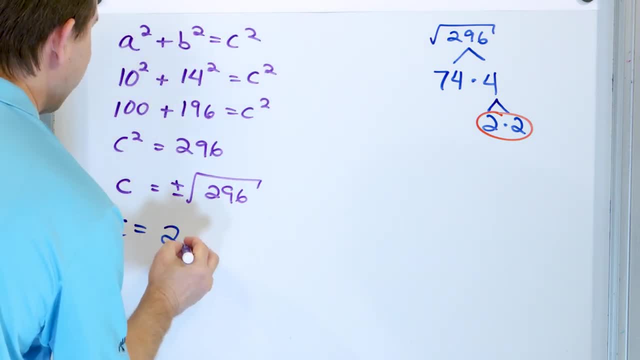 I guess I'll do it. maybe over here This single two will come out and under the radical will be the only thing left behind 74. And you can't really simplify that any further Now. it was plus or minus. I dropped the minus sign. 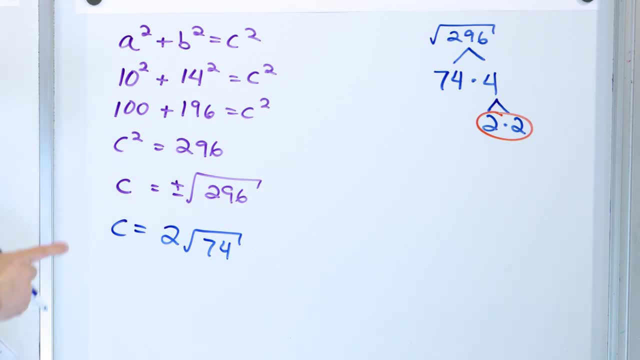 because there is no such thing as a negative length of a rope. okay, The units here were centimeters here and centimeters here, so the distance of the rope is all written in terms of centimeters, and this is the exact answer that you would circle on a test. 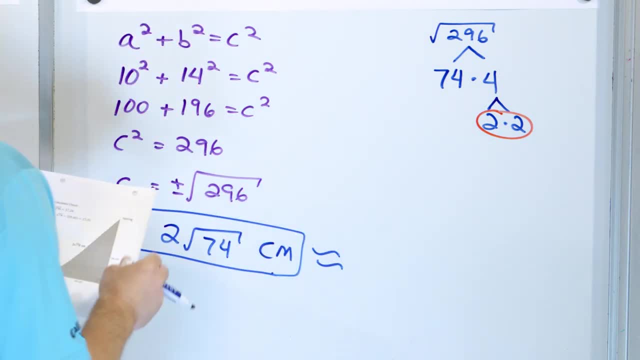 But you also know that this is approximately equal to when you dump it in a calculator in terms of a decimal, 17.20 centimeters. If you put 296 in a calculator and take the square root, you're gonna get 17.2,. 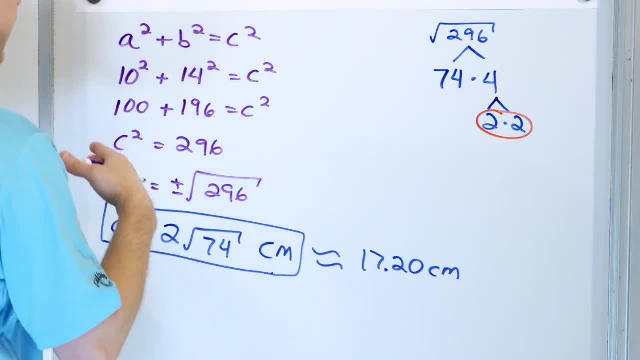 or once you round it to two decimal. it's gonna go on and on. you have to round it And if you do this, one square root of 74, you're gonna get 8.6. once you round it, Multiply by two, you're gonna get 17.2.. 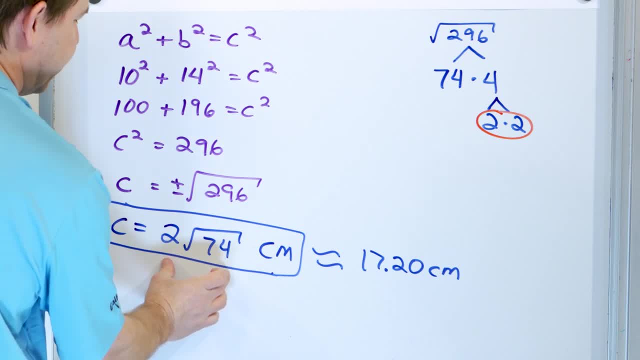 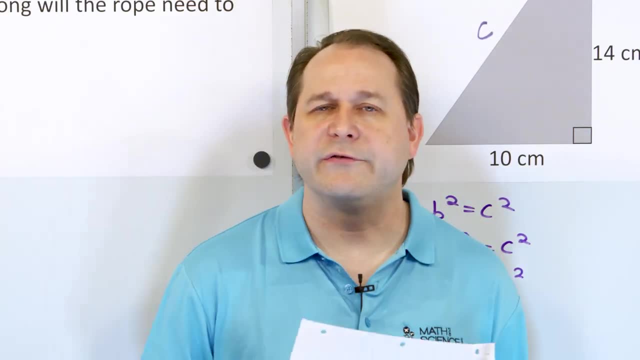 So these two things, even though they look different, they're exactly the same thing. This is more simplified. That's why we're circling two times the square root of 74 in centimeters for the length. So in this lesson we really wanted to do some problems.